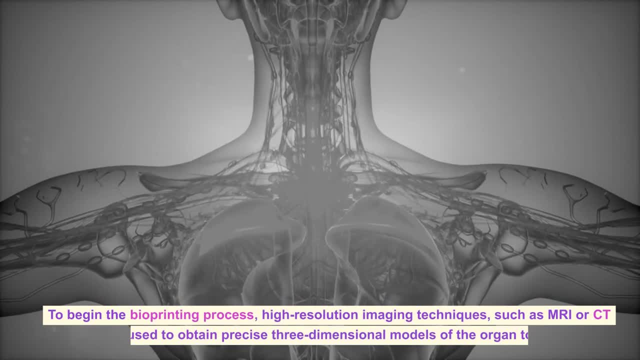 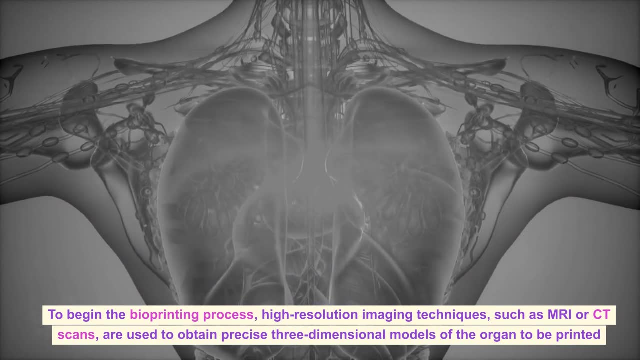 1. Imaging and Scanning To begin the bioprinting process. high-resolution imaging techniques such as MRI or CT scans are used to obtain precise three-dimensional models of the organ to be printed. 2. Selection of Bioink and Cells. 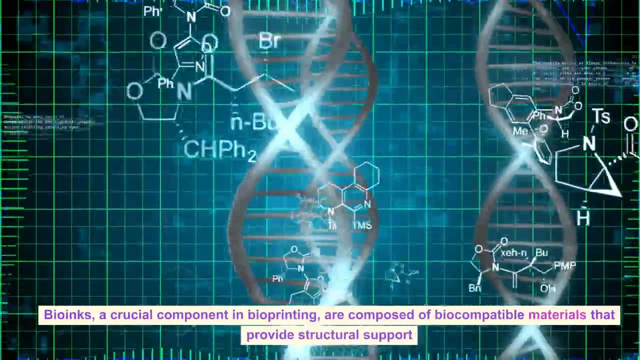 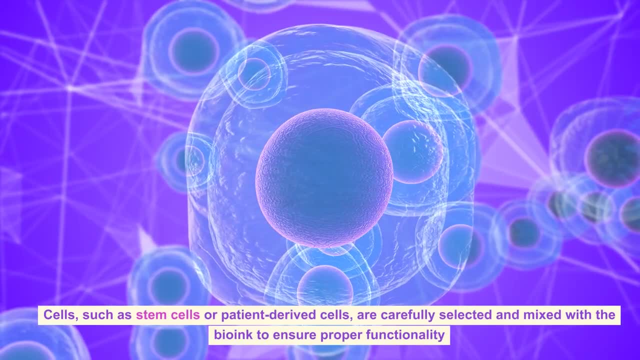 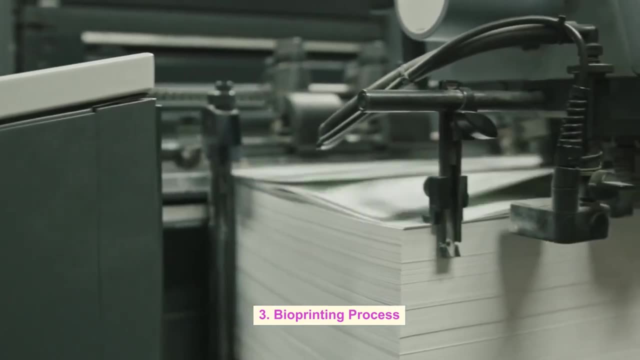 Bioinks, a crucial component in bioprinting, are composed of biocompatible materials that provide structural support. Cells such as stem cells or patient-derived cells are carefully selected and mixed with the bioink to ensure proper functionality. 3. Bioprinting Process. 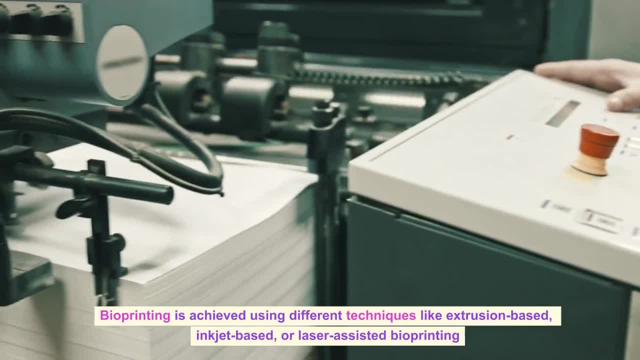 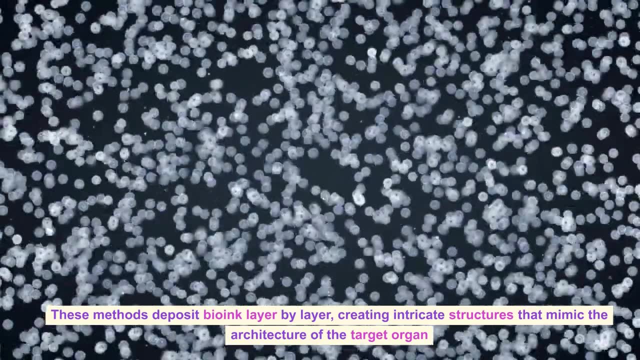 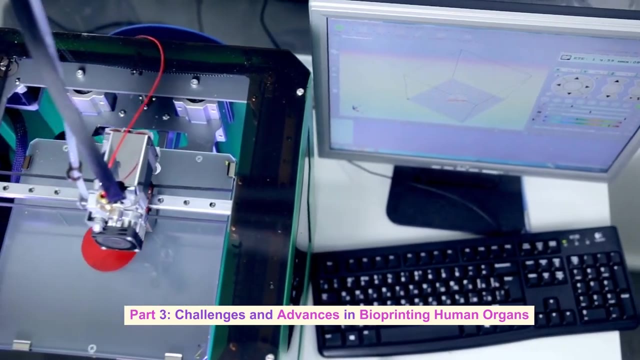 Bioprinting is achieved using different techniques like extrusion-based, inkjet-based or laser-based. These methods deposit bioink layer by layer, creating intricate structures that mimic the architecture of the target organ. Part 3, Challenges and Advances in Bioprinting Human Organs. 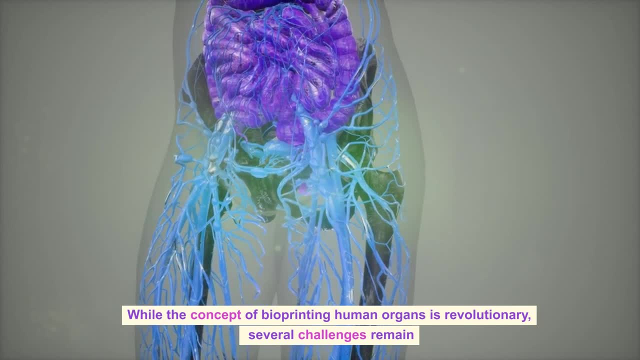 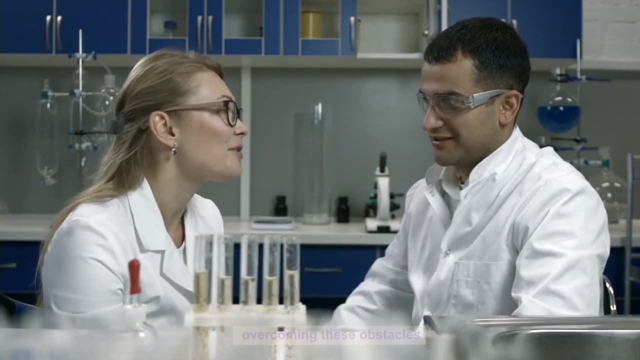 While the concept of bioprinting human organs is revolutionary, several challenges remain. However, researchers and scientists are making significant progress in overcoming these obstacles. 1. Vascularization: Developing a functional vascular network within bioprinted organs is crucial for 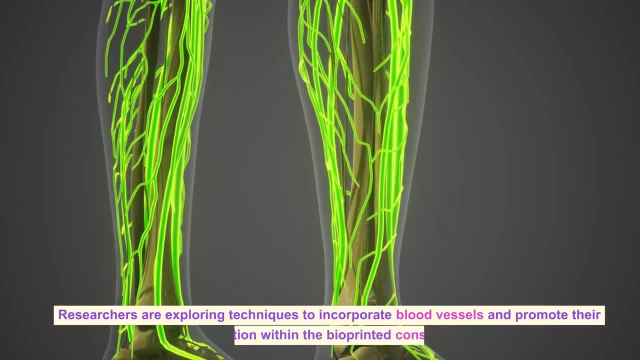 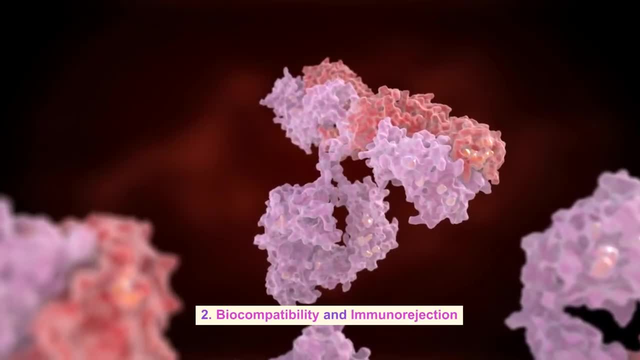 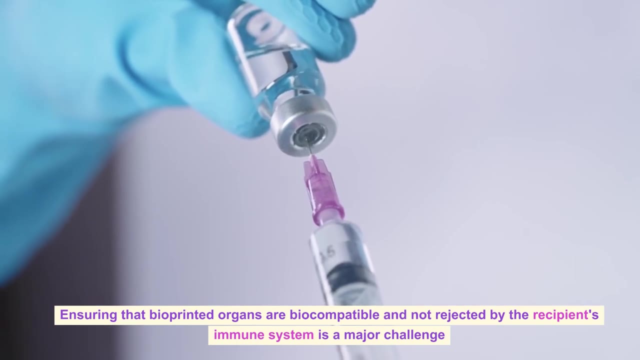 ensuring their survival and functionality. researchers are exploring techniques to incorporate blood vessels and promote their formation within the bioprinted constructs. two: biocompatibility and immunorejection. ensuring that bioprinted organs are biocompatible and not rejected by the recipient's immune system is a major challenge scientists are investigating. 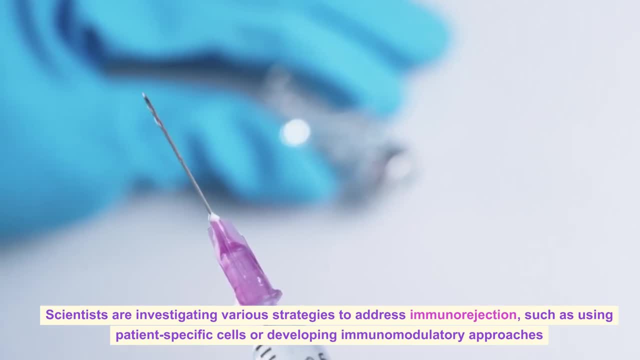 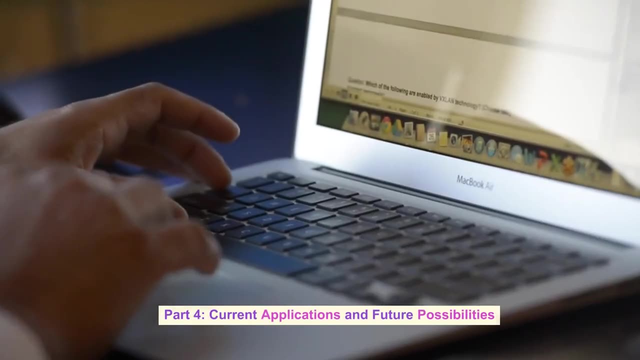 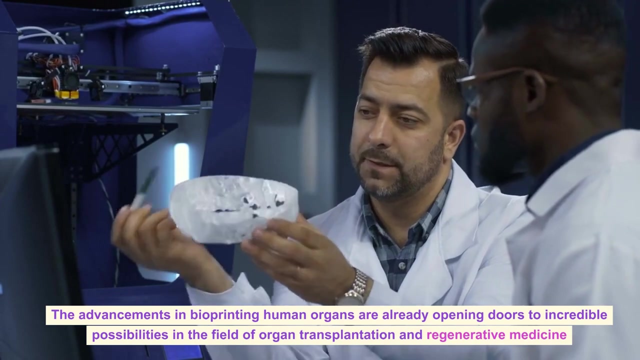 various strategies to address immunorejection, such as using patient-specific cells or developing immunomodulatory approaches. part 4: current applications and future possibilities. the advancements in bioprinting human organs are already opening doors to incredible possibilities in the field of organ transplantation and regenerative medicine. 1. organ substitutes for. 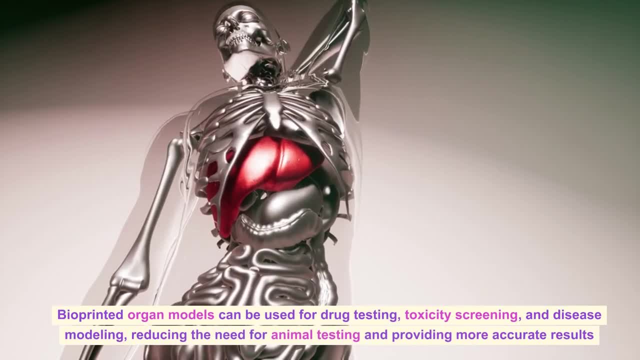 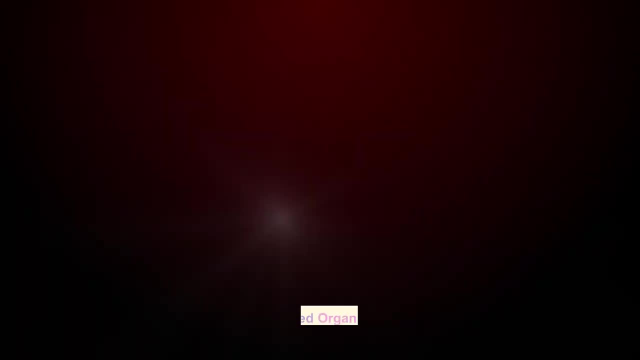 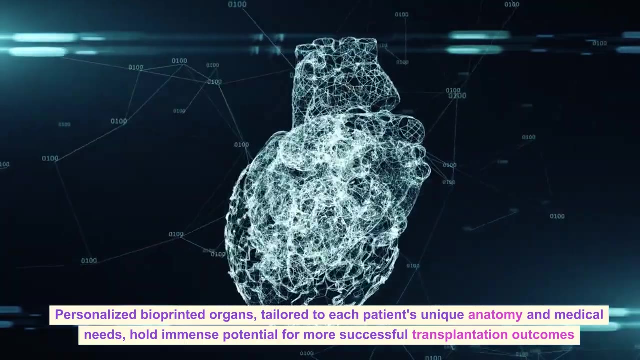 testing. bioprinted organ models can be used for drug testing, toxicity screening and disease modeling, reducing the need for animal testing and providing more accurate results. 2. customized organ transplants: personalized bioprinted organs tailored to each patient's unique anatomy and medical needs.